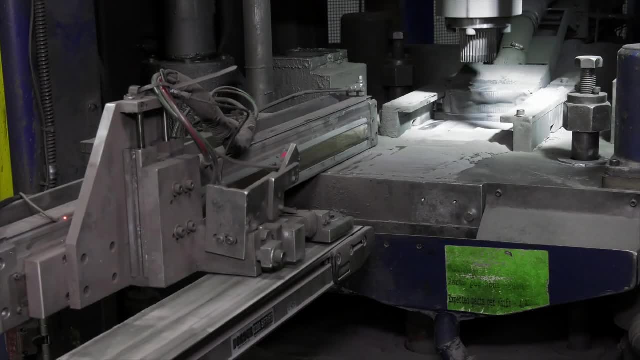 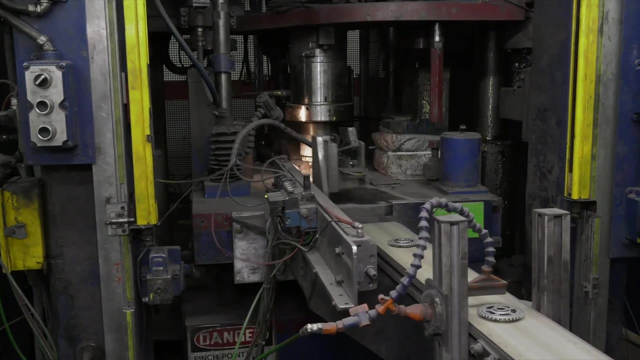 that you're looking for from the product are not going to be in that green part. but it begins with the shape. The PM process is kind of unique. You get a shape first and then you get a pattern, get the properties. The properties are all developed in that sintering furnace. So for 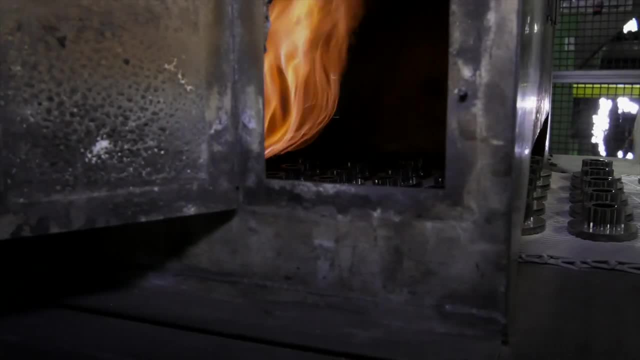 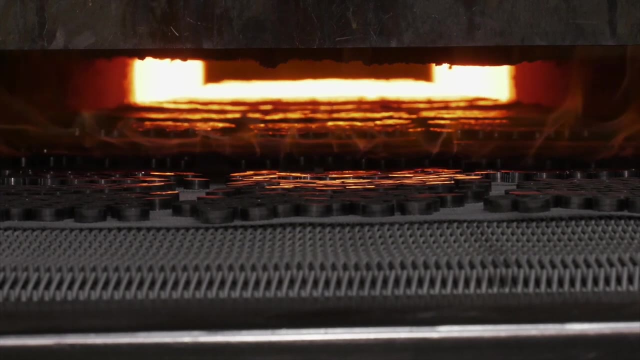 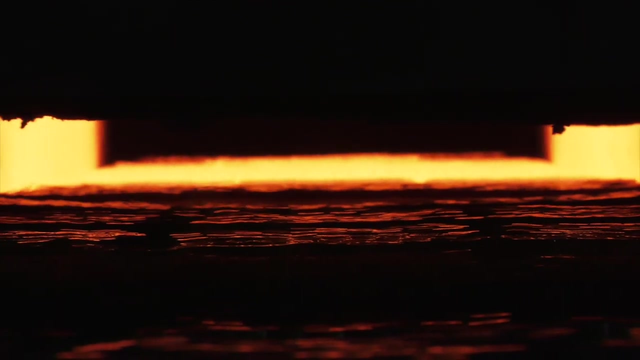 steel, we'll be in the 2000 Fahrenheit range or about 1100 degrees Celsius range. Certain atmospheres are used in the steel world. We use nitrogen as a protective atmosphere. Hydrogen is often used as a deoxidation or reducing atmosphere. It takes the oxides off all metal. 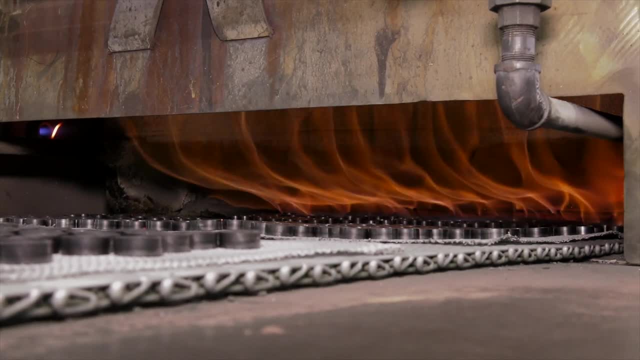 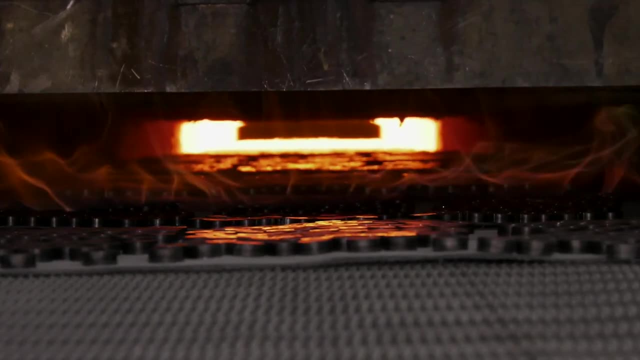 particles that have that oxide. We go through the sintering process and many, many things are going on. It's a fairly complex set of phenomena that occur in there, But one thing is first of all to: as we go in the sintering furnace, we take out the lubricant which is no longer necessary. 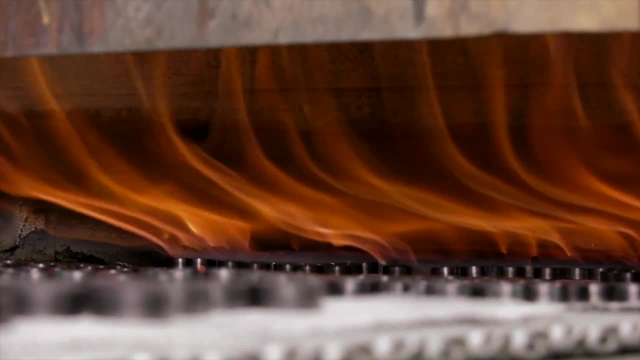 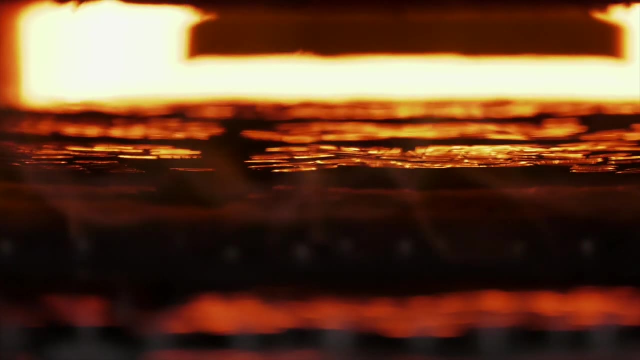 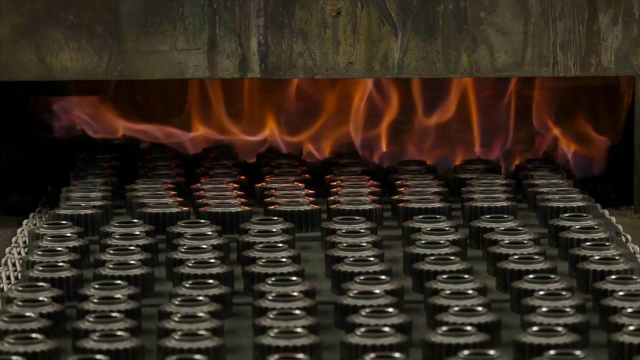 We only needed the lubricant so we could eject the part out of the dime. Now we have to take that lubricant out. That's done in the preheat sections of the furnace. as you go into the higher temperature sections of the furnace The temperature goes up and now we get actually particle to particle bonding. We also get 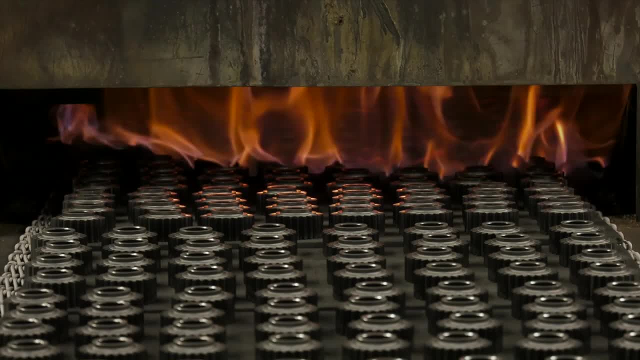 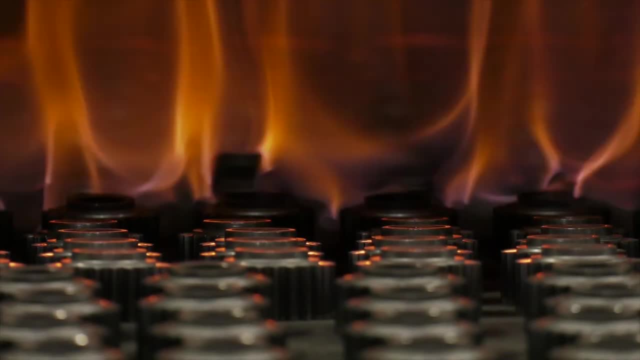 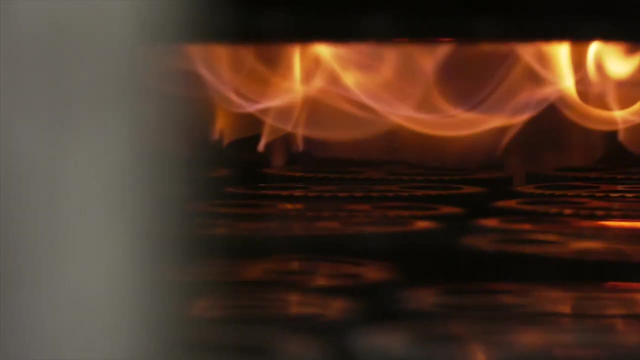 alloying from one particle to another, Different elements are maybe involved. The porosity is reduced. We will develop the strength that really is recognizable, that you need in the end product. So we're building the properties of strength at the sintering process. We also at that stage. 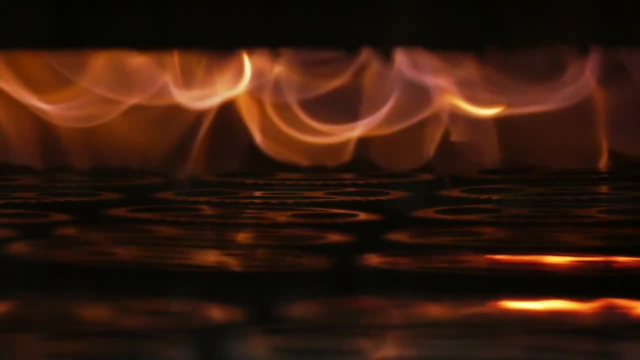 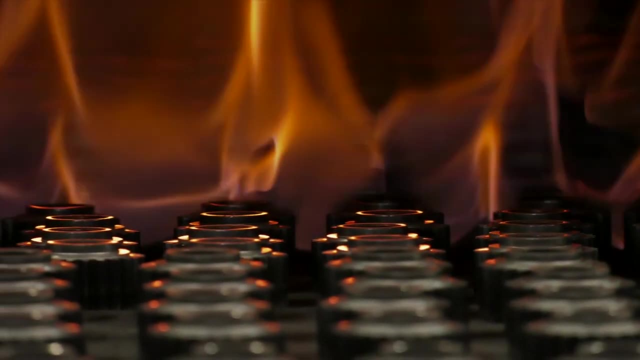 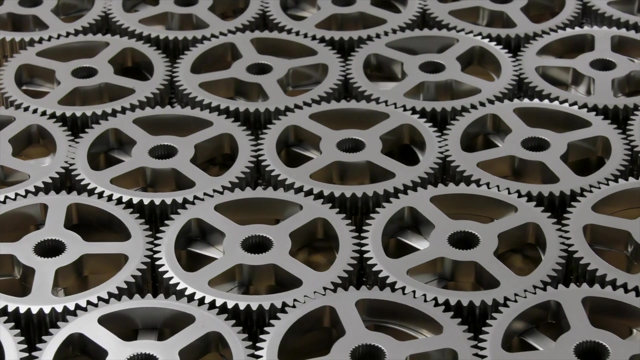 have quite a bit of control to ensure that we get the corrosion resistance that you need in the end application. if you're working with stainless steels, That product after sintering now has properties that you cannot recognize or differentiate between a hundred percent raw dense part versus a PM part, Unless, of course, you do. 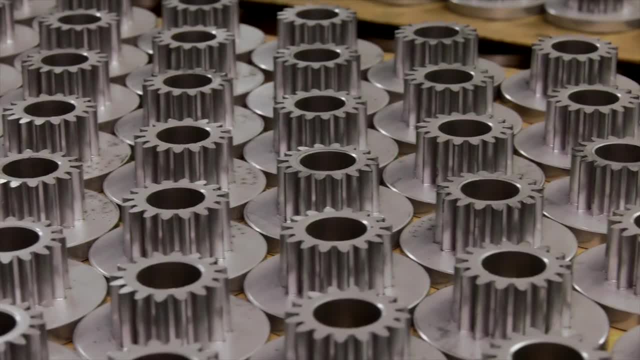 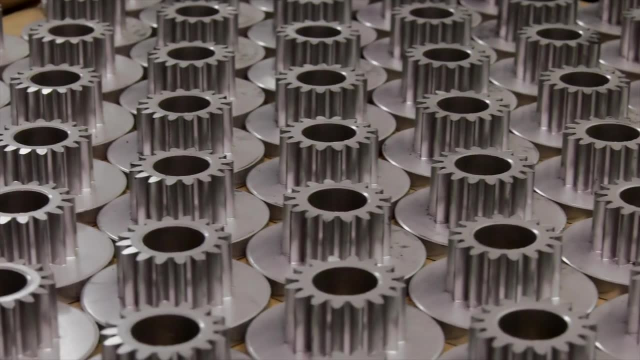 sections and then you'll see the porosity. But it has the strength that you're looking for and now it can go through all the operations that you might be able to do, The processes that you might take on for a 100% raw product, and that is heat treatment.